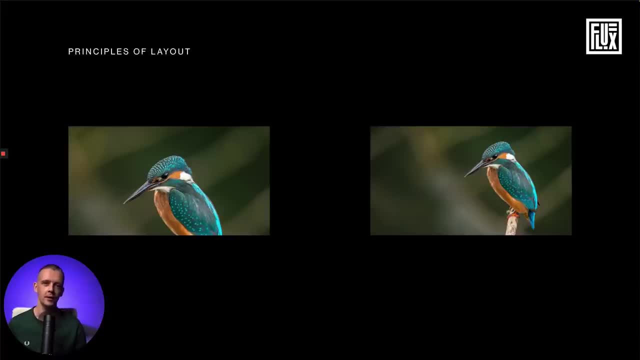 focal point is the rule of thirds, and photographers are taught to do this early. So in this image you can see that the bird on the left is placed in the centre. its head is placed in the centre of the frame vertically and horizontally, Whereas on the right not only can we see more of the bird, 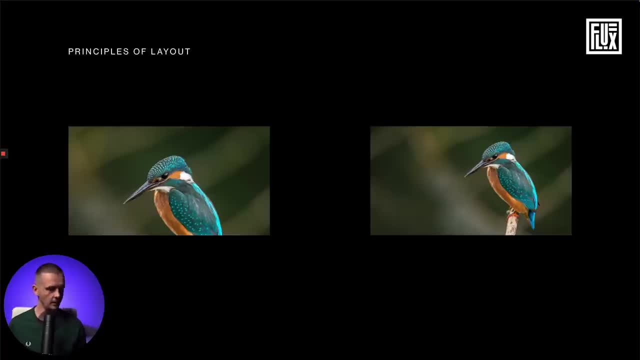 but the composition is more interesting because it is placed along these grid lines, so that its head, or kind of that point of weight around the neck, is placed in the top third horizontally and the right third vertically, And it makes for a more interesting, interesting image than the one where it's just in the centre. And you can apply this to layouts too. 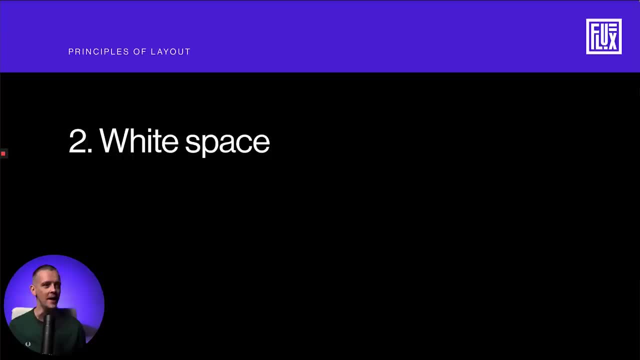 and we'll see that as all the principles come together at the end, But let me give you these quickly. Number two is white space, and this means quiet areas of visual rest which give you other elements, room to breathe, And we saw this in the photograph of the bird, The blurred out background. 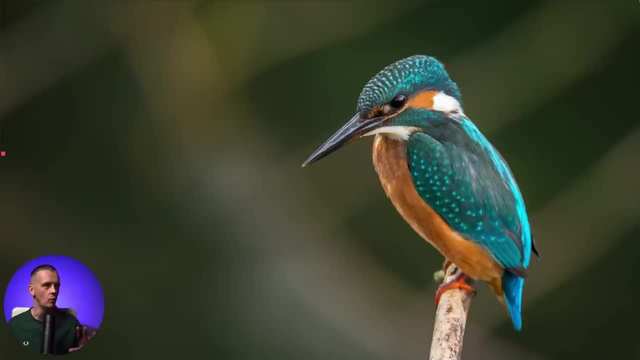 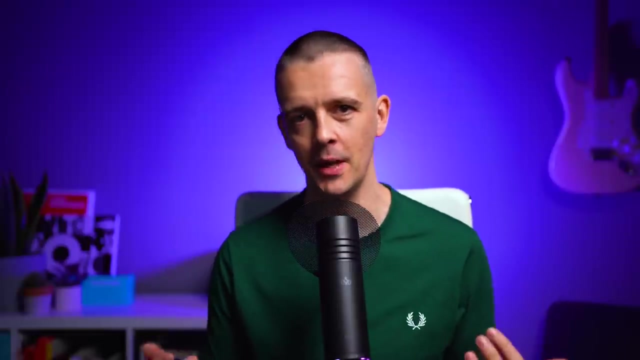 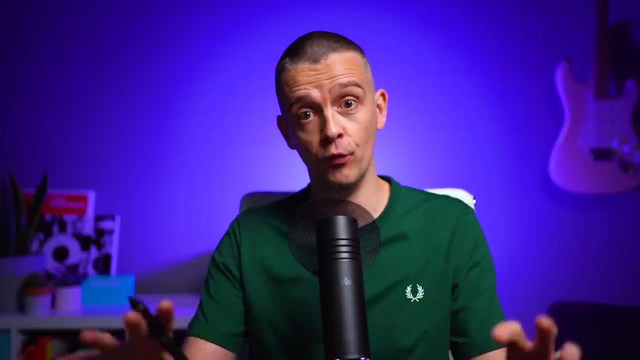 here provides the white space. White space doesn't have to be white, it just has to be a quiet area to focus on the part which is sharp and in focus, which is the bird itself. So just as music needs dynamics, that's loud and quiet, layouts need white space. The impact of the orchestra at full volume. 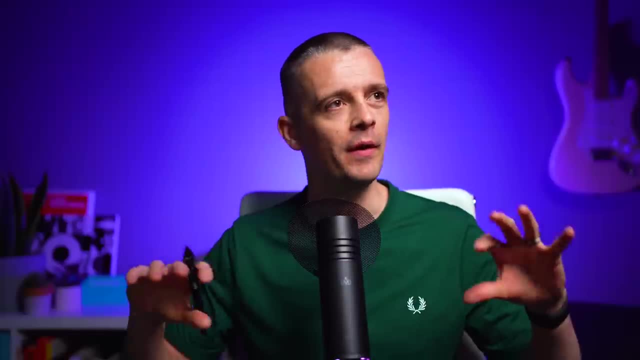 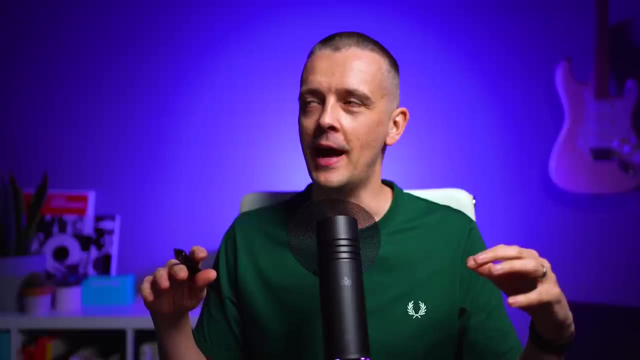 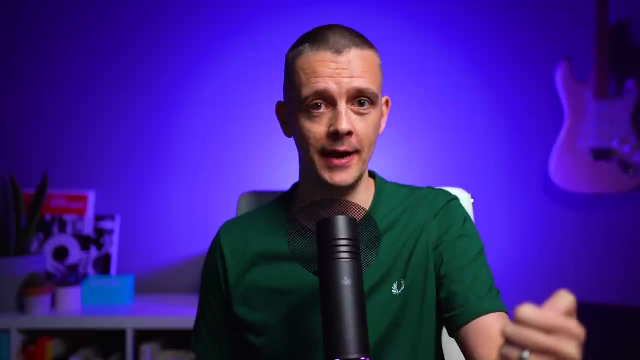 only works in a room where the acoustics are sufficient that the orchestra can play quietly and softly and we have that different feel. And then when they burst into life with an incredibly loud, powerful dynamic, it has that impact. And it's the same with a layout: Areas of quiet, areas of white space allow 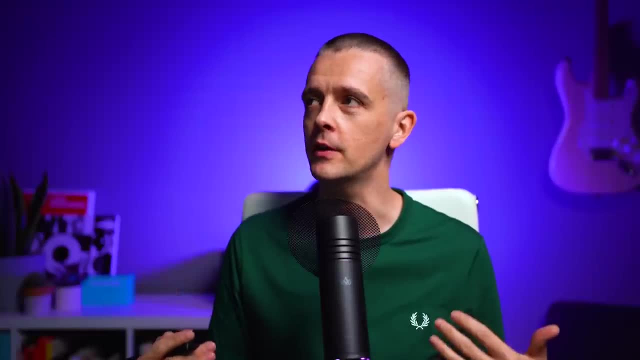 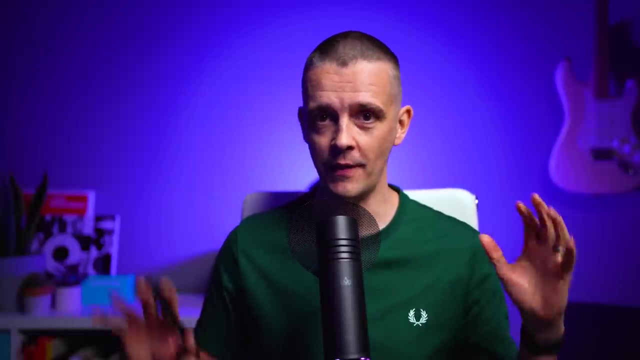 other elements to come to the floor and it makes them more interesting. It makes them easier to navigate around as well. And the third thing before we bring these all together is hierarchy. So this means giving priority to the most important elements. If everything's. 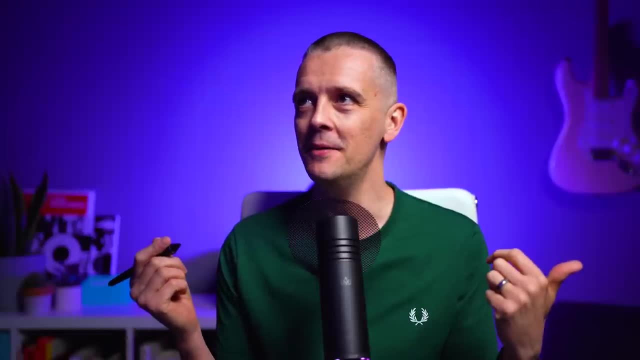 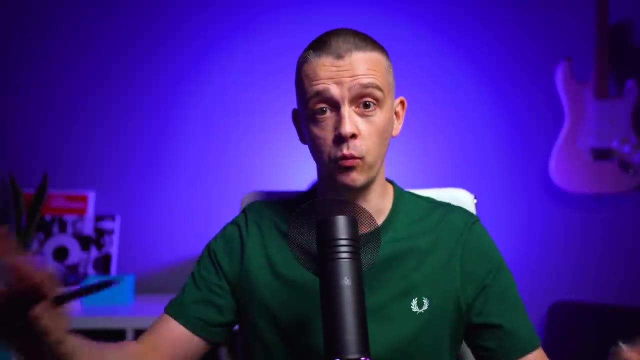 loud. if everything's on 10,- again like music- then nothing is emphasized. When you're mixing a track, you can't just turn up everything louder, It just makes a wall of noise. So some things have to come to the floor, like when you're listening to pop music. the lead vocals in the floor. 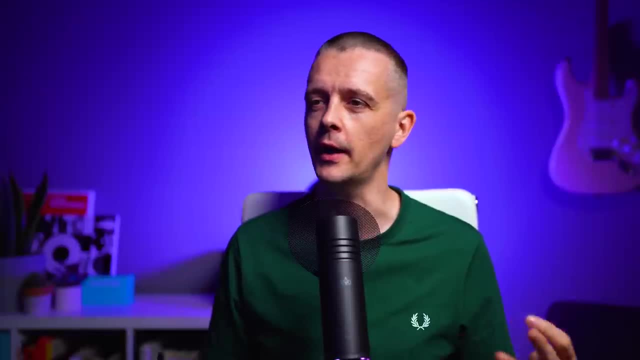 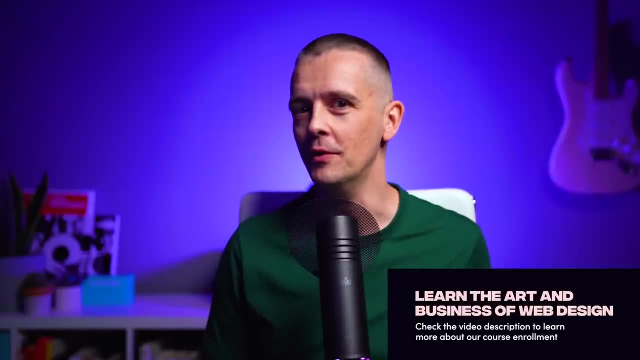 and some things have to be more to the background, a sense of hierarchy, And it's the same visually. Now this is design 101.. I appreciate that, But how often is this ignored in the real world? You want to orient your user. That means let them know where they are and then lead them on a journey. 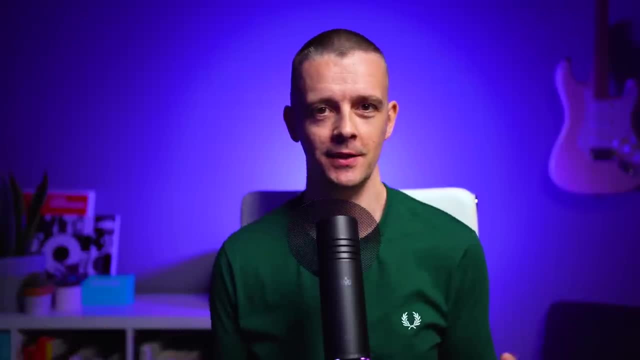 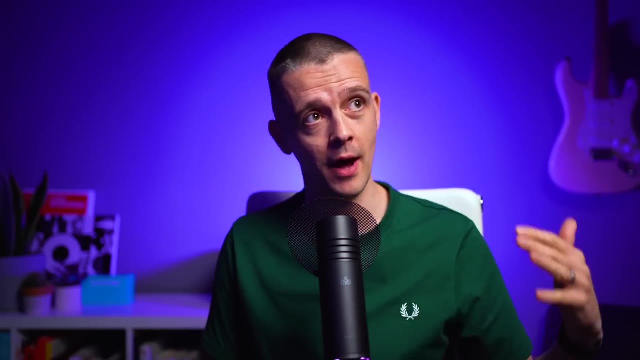 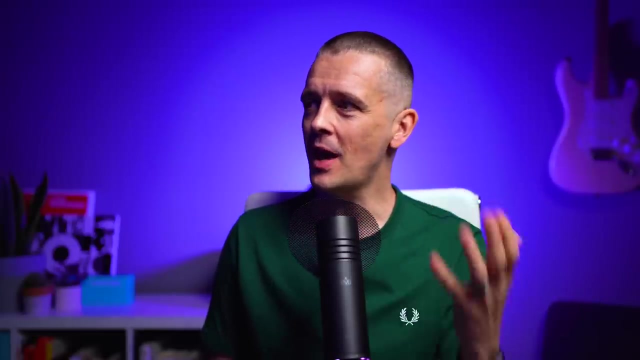 If you go to a map, maybe you're walking around a city as a tourist. the most important part is you are here, So they need to be oriented and be able to get their bearings of where they are, the layout where north is perhaps, and then where they want to go, And with hierarchy there's obvious things. 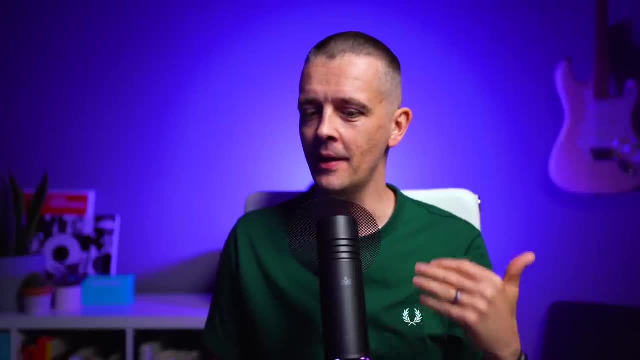 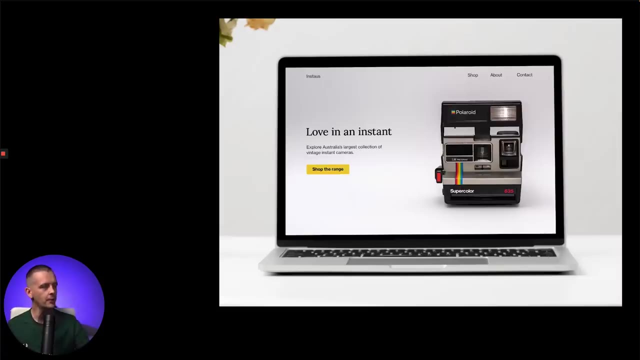 like, headlines tend to be more prominent than body copy, But let's have a look at some examples. So here on this hero section for this website, the dominant element, the focal point is the camera, And let's just annotate this: the camera here. So this is the dominant element, This is the 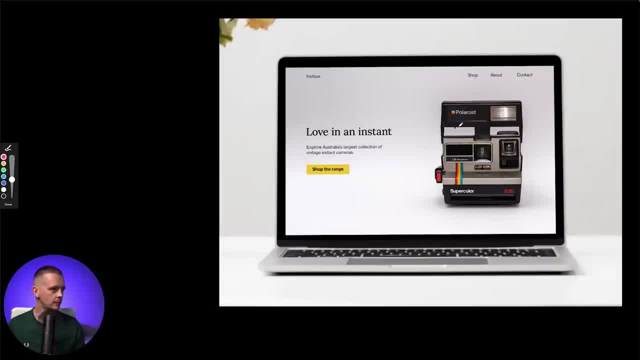 focal point And then there's plenty of white space around the image, but also around all the copy and such. So it allows you to, to to read it. It gives parts of rest within this, within the composition, And the headline here is clearly more prominent than the body copy. 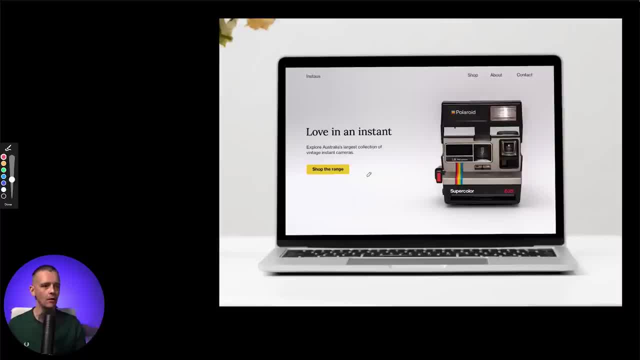 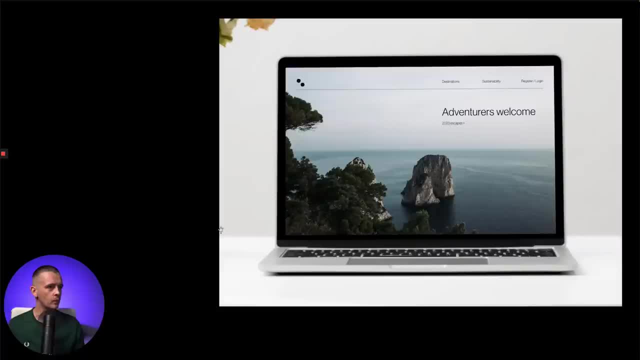 underneath, And so there's a clear hierarchy to it, as well as a clear focal point. So maybe with this next layout, similar with this next website again, So this time we don't have just a plain background: The photograph fills the entire background, However. 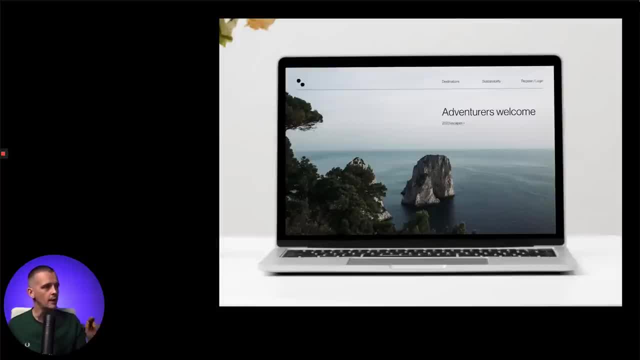 there's still clear areas of white space within this photograph. It's nicely composed So that the cliffs really stand out, because the sea and the sky give those white space areas. But then within the quiet areas there's been space to place the logo, the navigation, the headline. 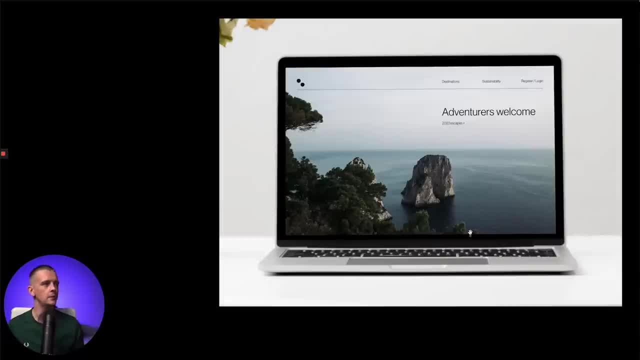 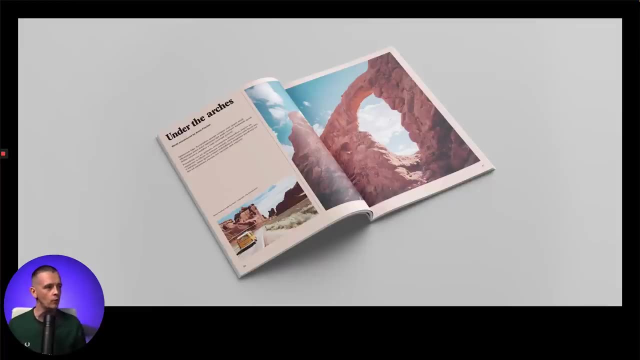 and the call to action very clearly. So we see this image, we get this feel, and then we read the headline and it gives us a sense of the kind of website that we're on straight away. Similarly with this magazine layout, we see first of all the focal point, this big photograph which spans over from the 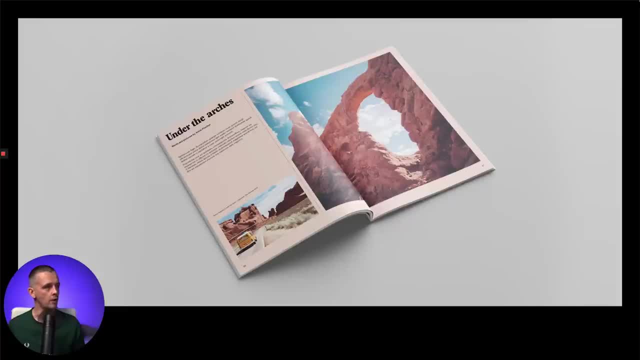 right onto the left page of this arch And as you're flicking through the magazine, this catches your eye as an eye-catching focal point for this photo essay, So it's going to lead you into that. So you see the picture and you get a sense of this is going. 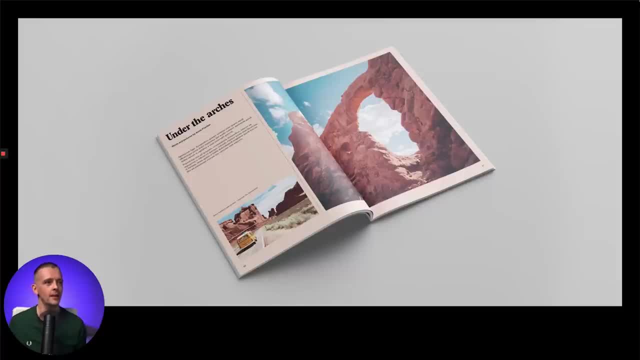 to be something from this American wilderness, which it is. Then the headline: it's clearly more dominant than the body copy, And there's also areas of white space. Not every cell within this grid has to be filled, and that gives chance for there just to be more of a sense of rest. 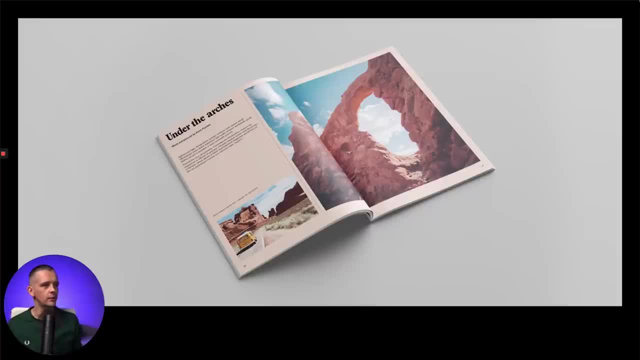 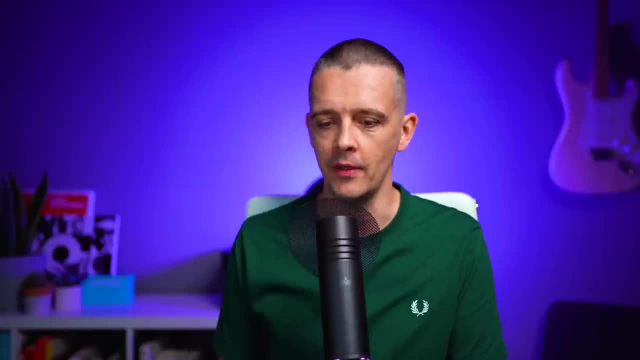 and it gives it more of a premium, relaxed feel to it as well. Now we can see this. These are made up examples that are quickly put together, but you want to train your eye so that you are aware of these principles while you're looking at them. So you want to train your eye and be so that you are aware of these principles while you're looking at them. 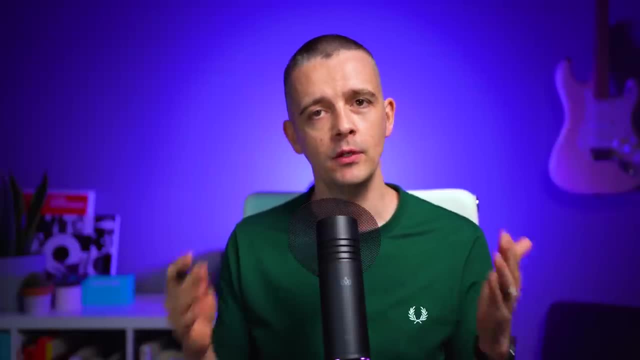 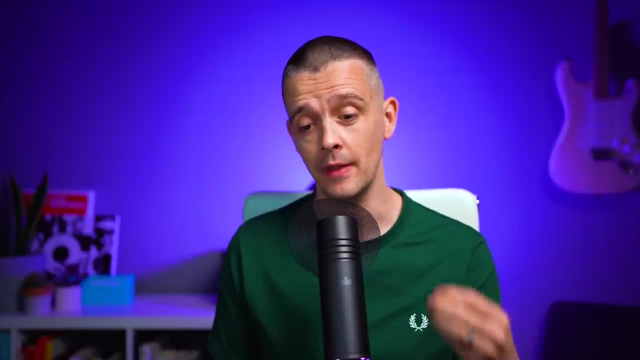 you want to train your eye and be, so that you are aware of these principles while you're looking at them learning, And so that, when you look at a layout, you can see them at work and you can understand why a skilled designer made the decisions that they did. So let's look at some real world. 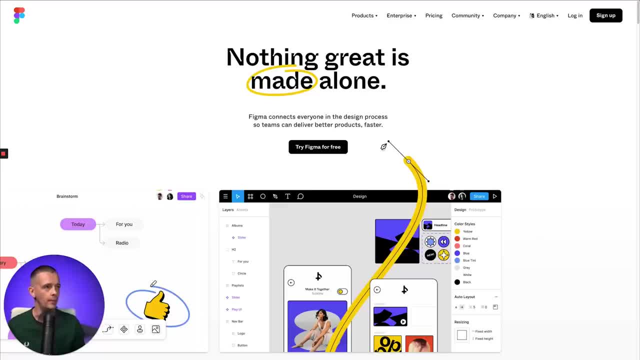 examples. So this is the hero section on the Figma homepage. So straight away we see the headline. it's at the top, it's big, it's bold. Now I've got a massive 5k screen here, So we see quite a lot. 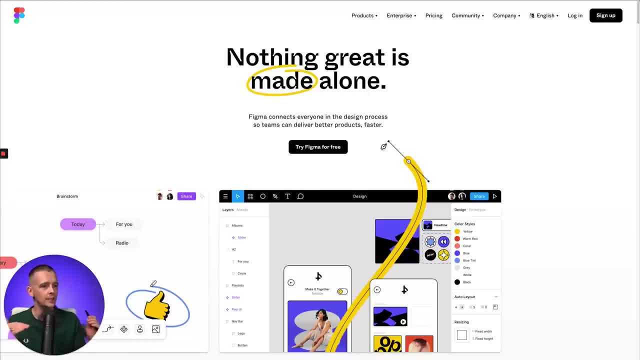 of the image, but maybe on a smaller screen. you just see a little bit of the screenshots here at the bottom below the full. but we see the headline and there's plenty of white space around it And things are sensibly placed and they're not crowding each other. So we get the concept of 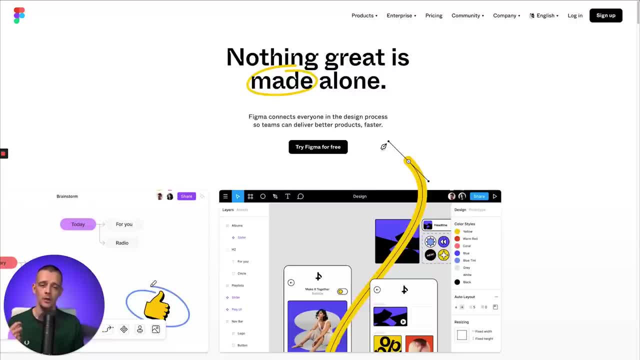 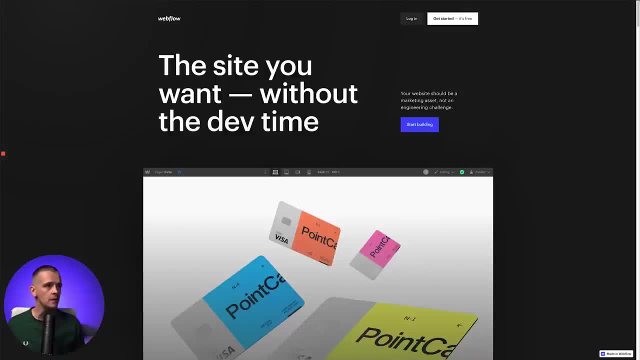 what Figma is about. They're making their unique selling proposition the collaboration aspect. So that's very clear at the top And it leads us down through this. Same with Webflow, very similar. They have a headline with Figma. it was black on white here. 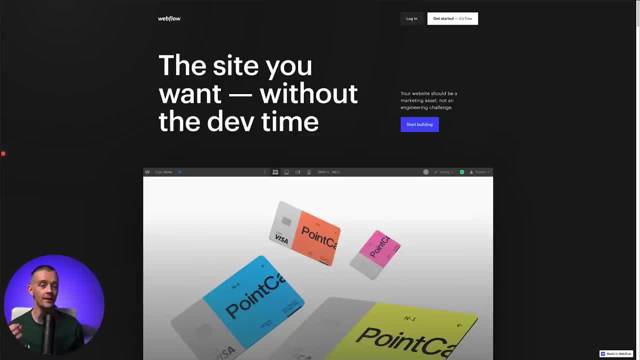 with Webflow. it's white on black or very dark And that's very clear and it's not crowded out by imagery. The site you want without the dev time. their value proposition is very clear and their logo is appropriately small. There's enough clear space between. 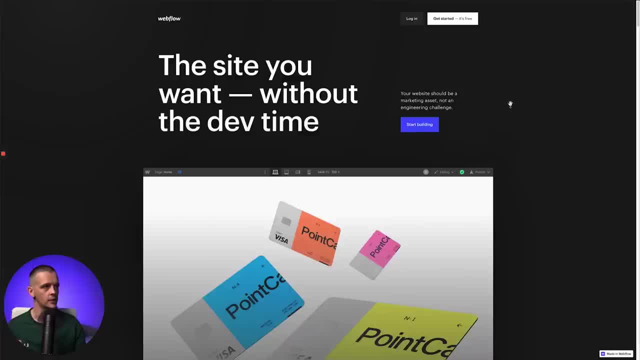 they make their navigation very simple as well. It's just a login or register so that you are drawn to the site. So that's very clear. These key elements, and they're able to get across their value proposition before encouraging you to scroll down the page, thereby showing you within the app. 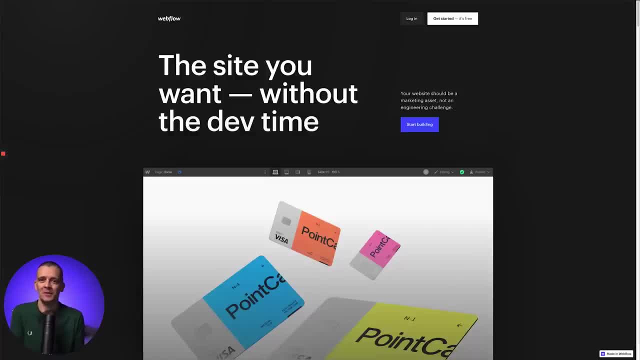 Now you're probably thinking: these are both in the design community. Of course they're going to have great websites and, more importantly, they're going to observe, just like, very basic principles of design. But what about the Pantone website? I mean, what is going on here? 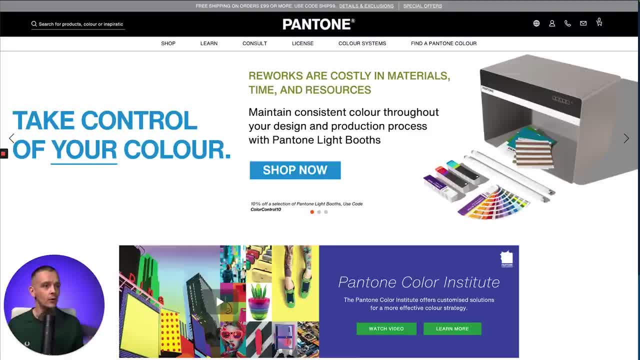 I come here and I don't know where to look. There's so much going on. I've got to work. I've got to force myself to look around to figure things out. What is the focal point here? Perhaps the light booth over on the far right? 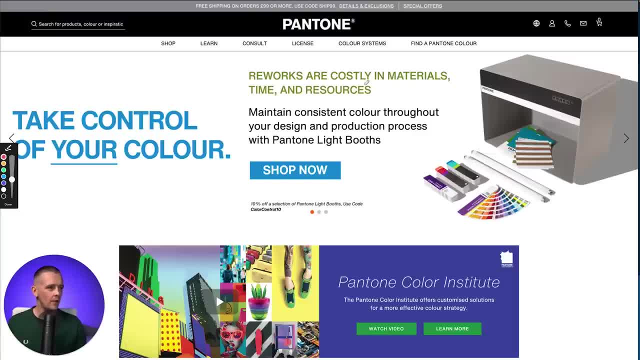 It could be this, but we've got this type in the center, So that's like in the center at the top. So I'm sort of drawn to that, But then the biggest headline is here, So I'm not really sure. I'm kind of all over the place And this hero section. 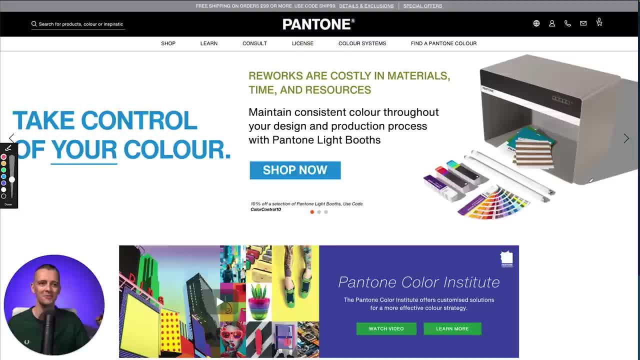 which is actually a carousel. So these are rotating, which will distract you even more. So I've decided to take a screen grab for you guys. But then below we've got like a big solid rectangle here. So this is very heavy And this has got like one to 10 images in the thumbnail. 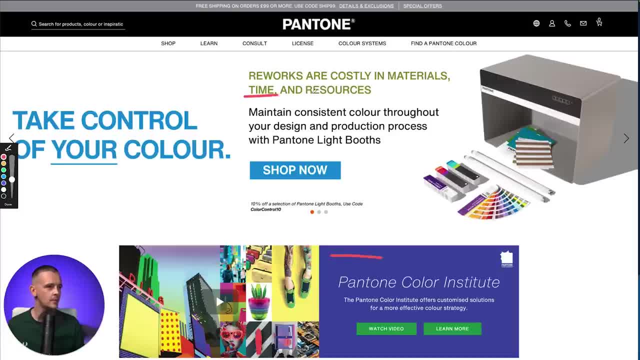 for this video. next to something on a colored background, I mean this type's in all caps and colored up, Two things that make type harder to read. Just so much going on. So I'm going to take a look at this. I'm going to take a look at this. I'm going to take a look at this. 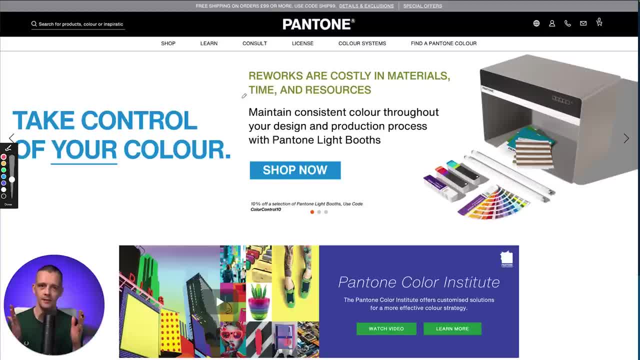 It's close to this now, so it's competing. So if they would just go back to these very basic principles- focal point, hierarchy, white space- If they were observed and Pantone's value proposition and the sense of their brand came across- I mean, this is a brand for designers. 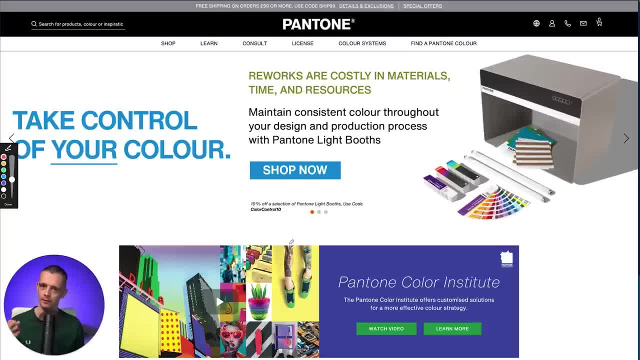 exclusively Fashion designers, interior designers, graphic designers. So it needs to look good, It needs to feel good, And Pantone do a really good job with their products and their merch and that's not coming across in their website And, yes, they have.